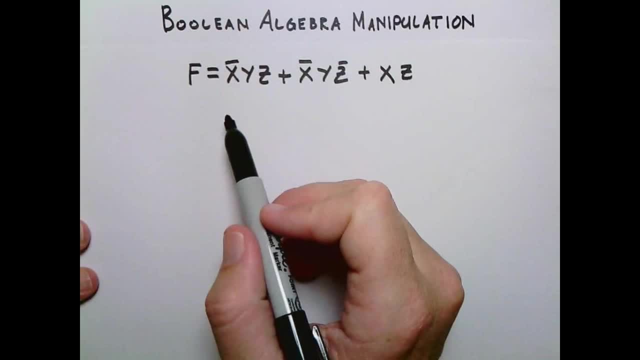 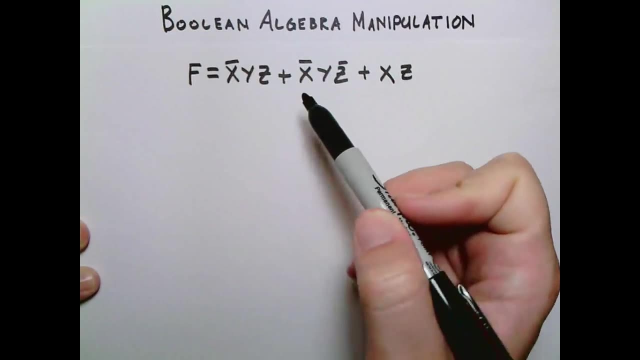 So let's do this one. It's kind of a simple example And basically, when you're doing this analysis or this manipulation right, the things you need to look for are places where things sort of repeat themselves in the equation. So, for example, we can see here that we've 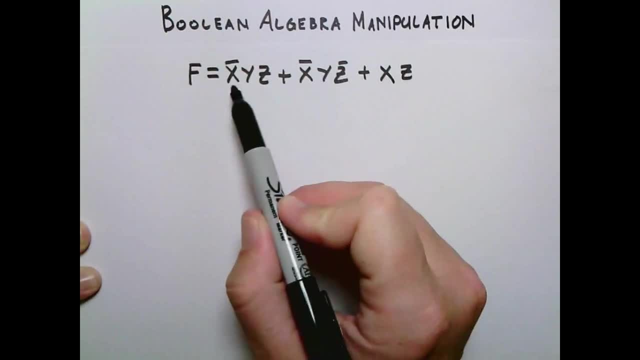 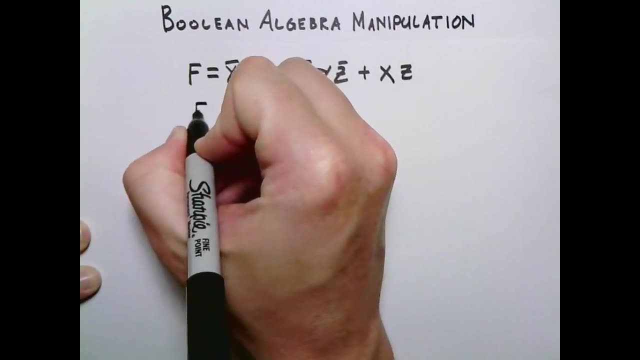 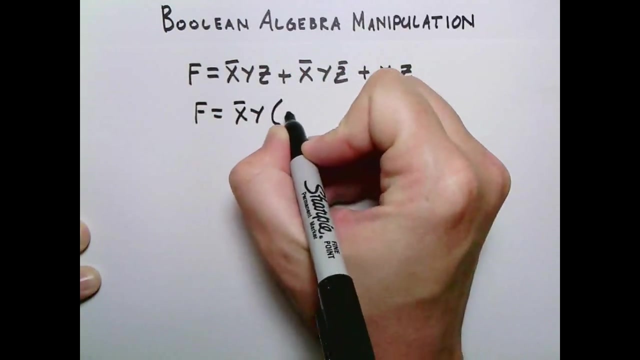 got not x and y and not x and y here in both places and z and not z attached So we can use the distributive property. We'll say f is equal to, not x and y, Mussp to plus x or not xay z. 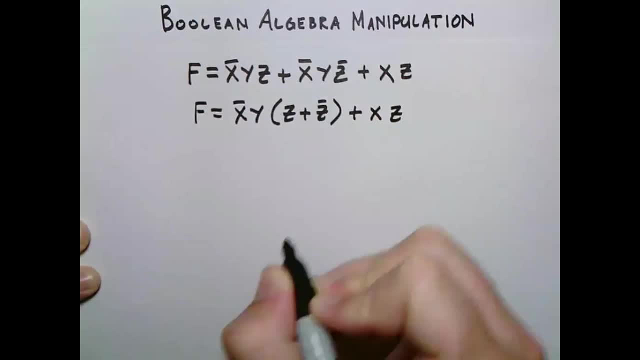 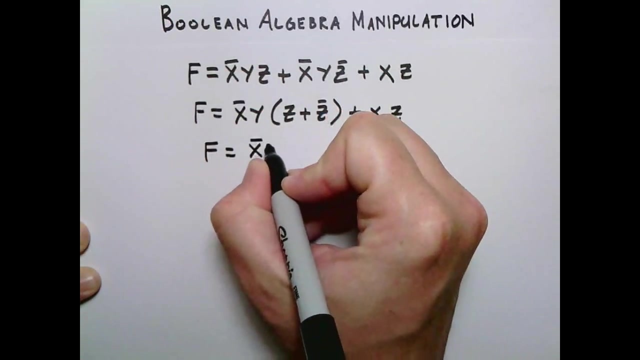 to pull out the not x, y, not x and y and z, or not z plus x, z. So, and if you remember from our Boolean algebra identities lesson, we know that anything or-d with its compliment is equal to one. So f is equal to not x, y and 1, or x and y. 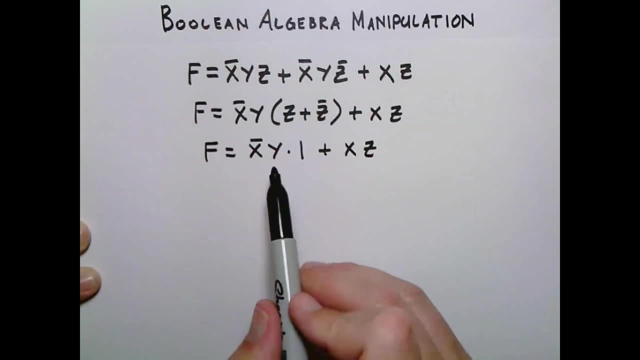 f is equal to not x, y and 1, or x and 1.. Then we have x at getting the one we wanted, XZ, and remember the identity: anything anded with 1 is going to be itself. So F is equal to not X and Y. 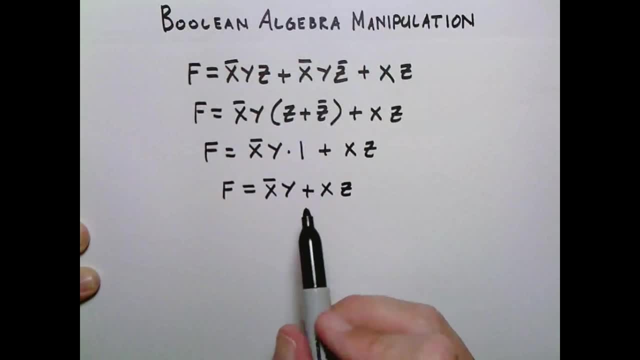 or XZ. So when we look at this, there's really not a lot else we can do. We've got X and not X, but we've got Y and Z. So this is about as simple as this guy can get, So we'll leave it right there. So let's just recap this: 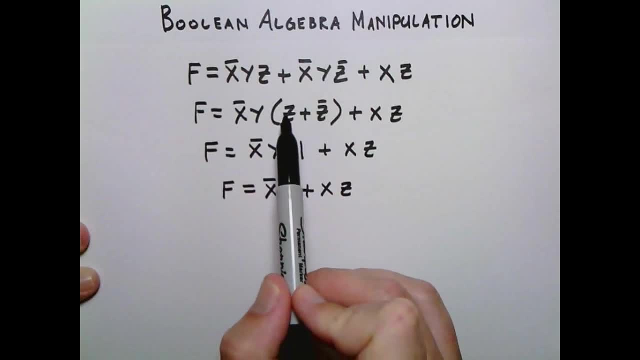 example, We took not X and Y, we pulled it out, leaving us with not X and Y and Z, or not Z, which simplified to 1, and not X and Y, and 1 is just equal to not X and Y. So we were left with F is equal to not X and Y, or. 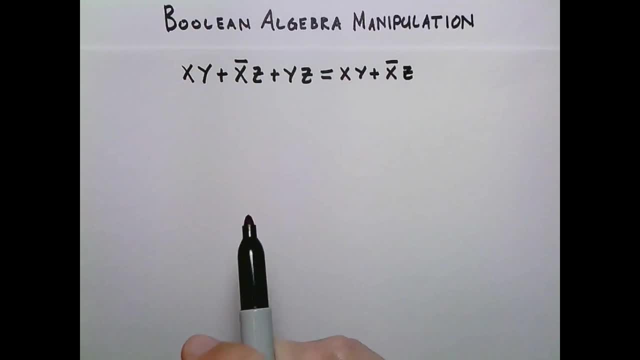 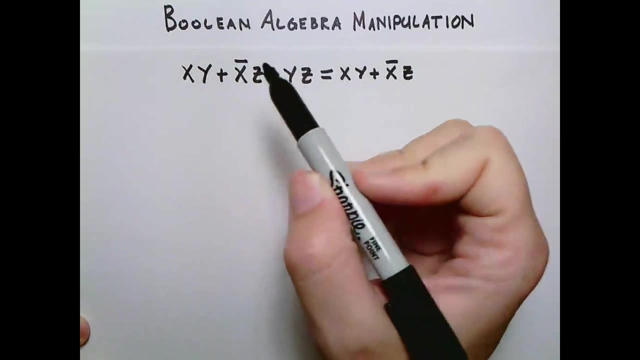 X and Z. Okay, so that was pretty simple. Let's do a slightly more complex example. So here we're just going to do a Boolean algebra proof. We're going to look and see and show that X and Y or not X and Z, 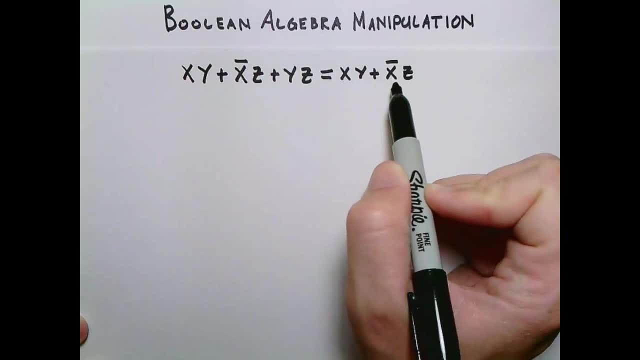 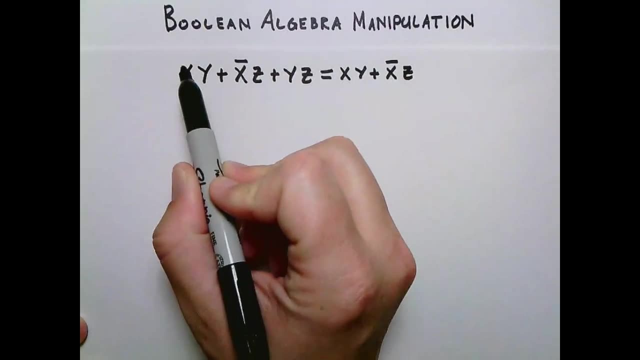 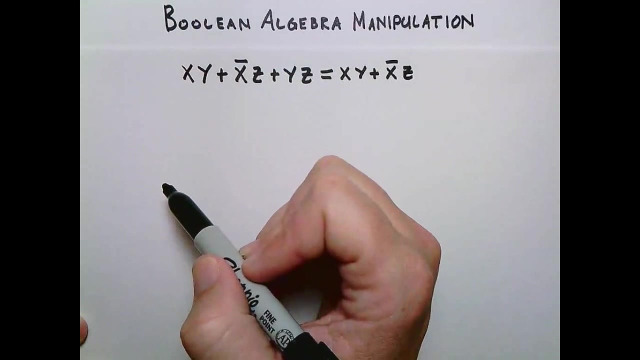 or YZ is equal to XY or XZ, So let's dive right in. So I always like to start with manipulating. I like to start with manipulating the more complex side, right, because it's easier to reduce than it is to sort of build things out. So 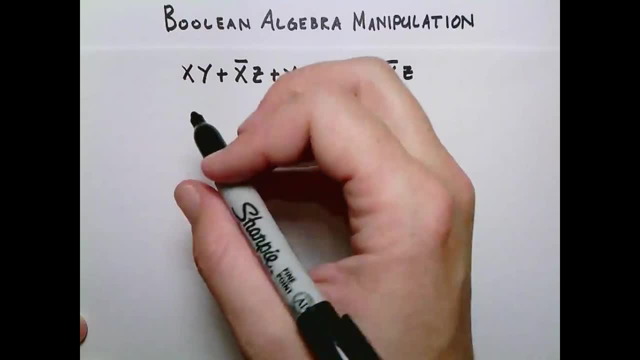 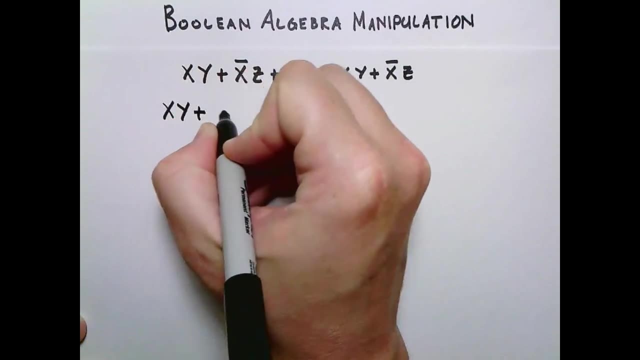 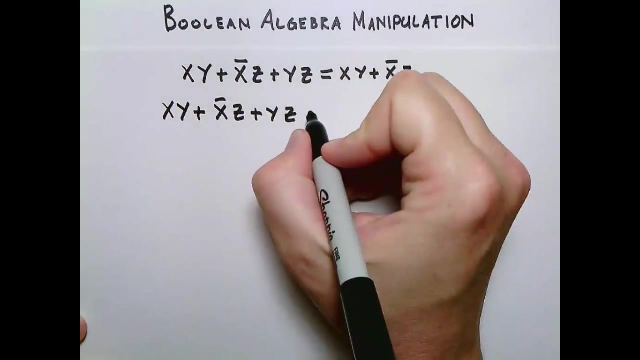 let's go ahead and jump into that. So let's see, There's a couple ways to do this, but let's go about it this way: We're going to say X and Y, or not, X and Z, or Y and Z equals, and we'll just kind of keep everything going. 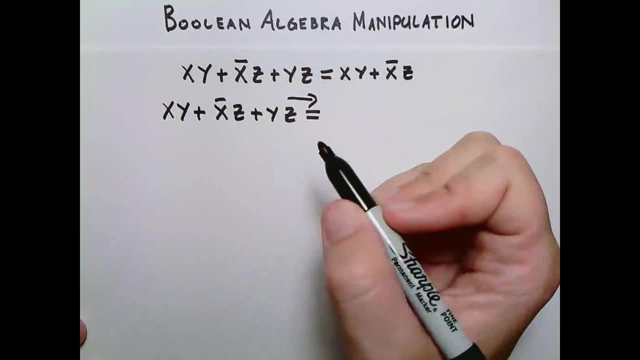 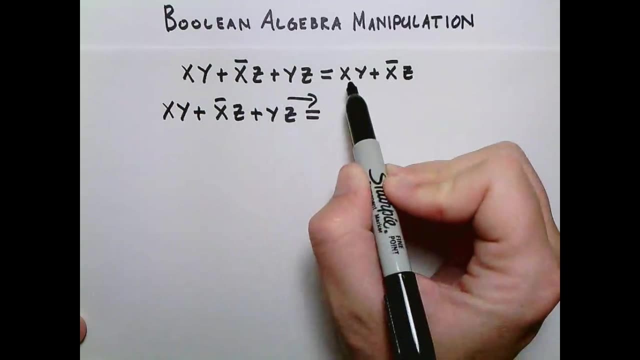 on the right side here and triple down. So when you want to look at this sort of thing, the first thing is say, well, what is in the side that we're trying to get to right? We're trying to make this side look like the right side. Well, this side's got X and Y. 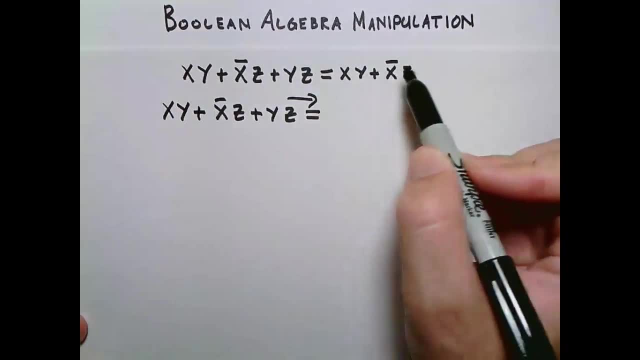 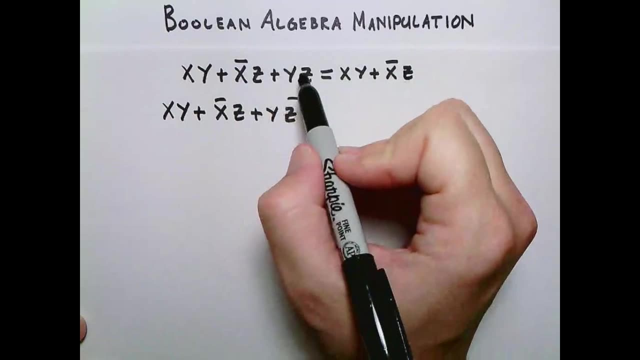 and so we've got X and Y here. that's cool. We've got X and not X and Z, so that's there. that's cool. So we actually already have the, the expression that we're trying to get to, in our side. All we need to do is get rid of. 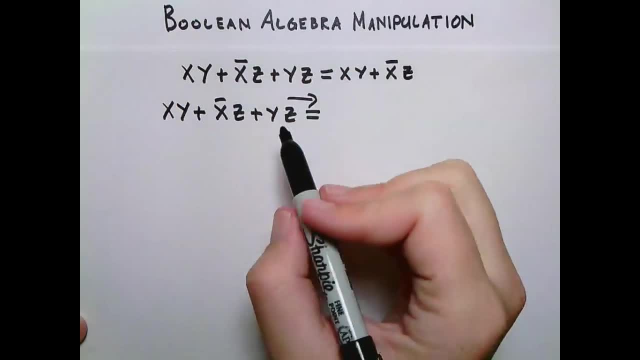 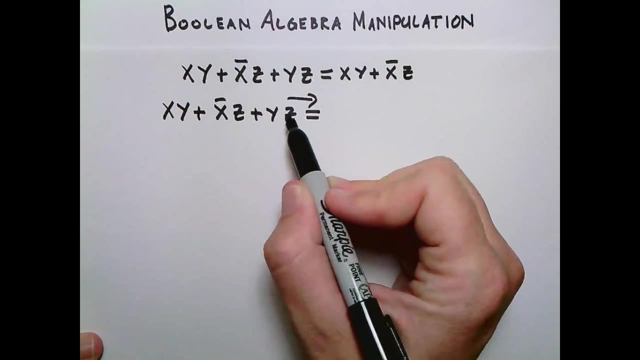 Y and Z, and it's actually. there's a pretty easy trick to do this. So the first thing you do is look at what you're trying to get rid of and notice, well, what input is not present in this little Boolean expression, right? 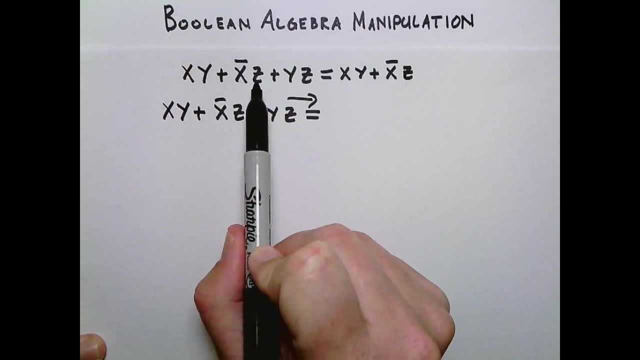 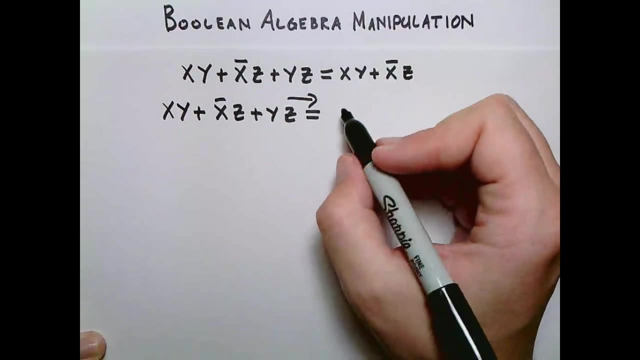 So this system has three inputs: X, Y and Z, and here we just have Y and Z, no X, right? So to get rid of this guy- it always seems to work out that you can do this. Let's write the other parts, X. 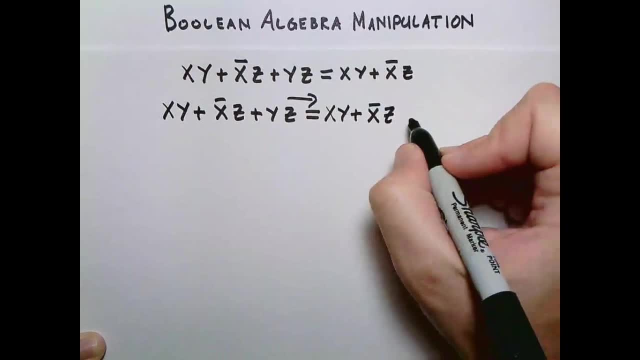 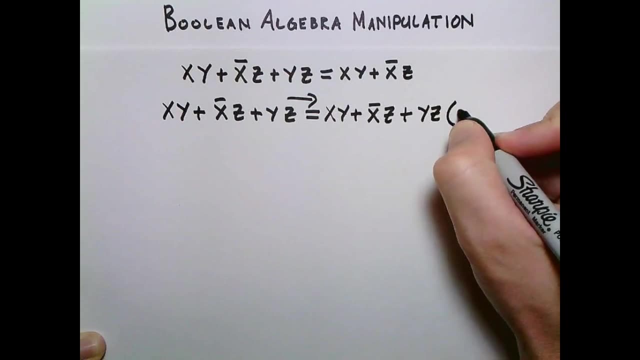 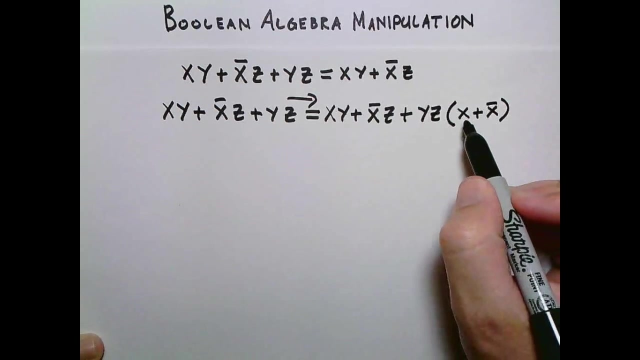 and Y, or not X and Z, or Y, Z, and end it with the input that's not present, but it or its complement. So we're going to say and X or not X, because, remember, anything or its complement is equal. 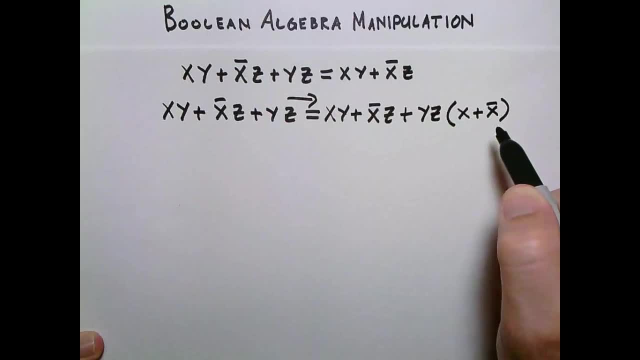 to 1, right, So we're just ending by 1,, which is itself. so we're actually not violating the equation, right? Take it back to high school algebra. we're multiplying by 1.. So once we have that, we can use the. 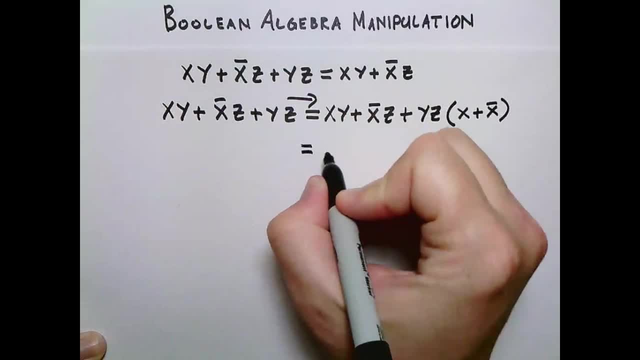 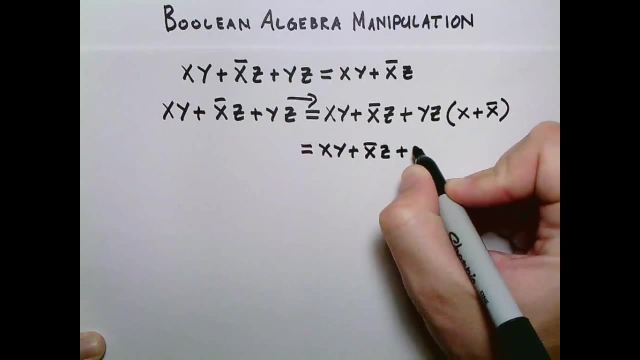 read of property to bring Y Z into this guy. so we're going to have X Y or not X Z, or X Y Z or not X Y Z. So now we want to look and see what stuff we can get rid of. 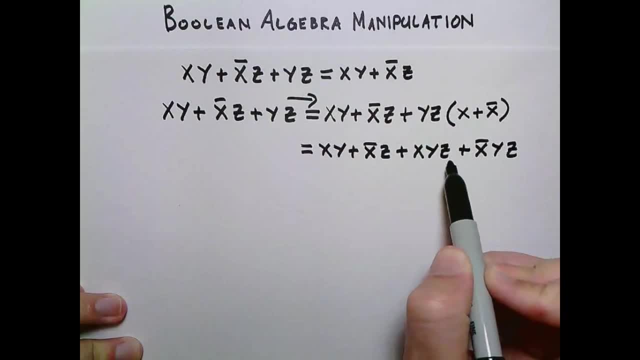 So we've got X and Y and X, Y, Z over here, so let's group these guys together. Remember, we can shuffle these things around and that's not violating any of the rules. So X and Y, or X and Y and Z. 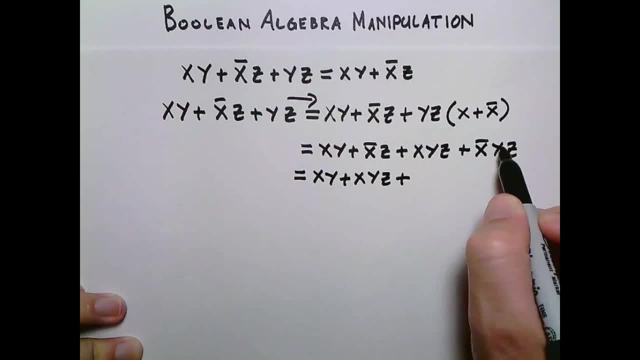 or, and here we have not X and Z and not X, Y and Z, right? Remember, we can move these guys around too. so we've got, let's say, X, not X, Z or not X. 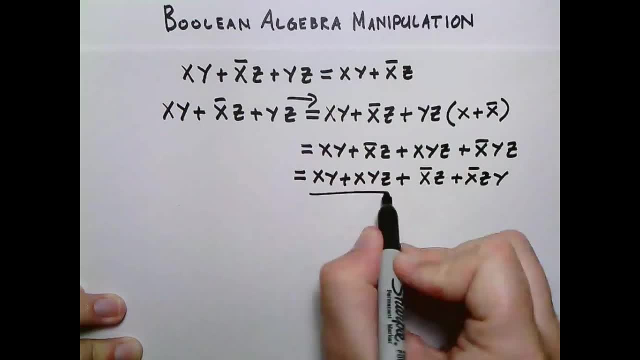 Z and Y. So in both of these cases we can take the distributive property to pull the common terms out. So we're going to have X, Y and 1,, 1, or Z or not. X, Z or. 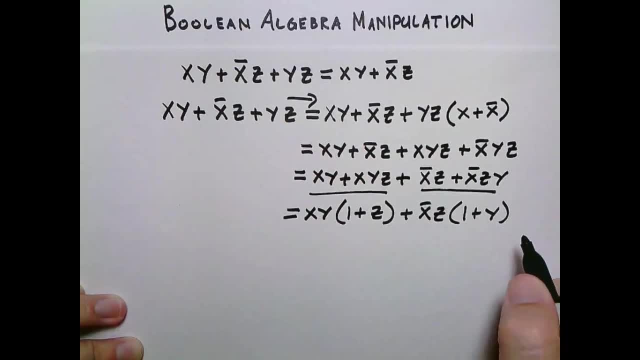 1, or Y, excuse me, and 1, or Y. So, and we know that anything or-ed with 1 is just equal to 1, so these guys cancel out to 1, so we have X and Y. 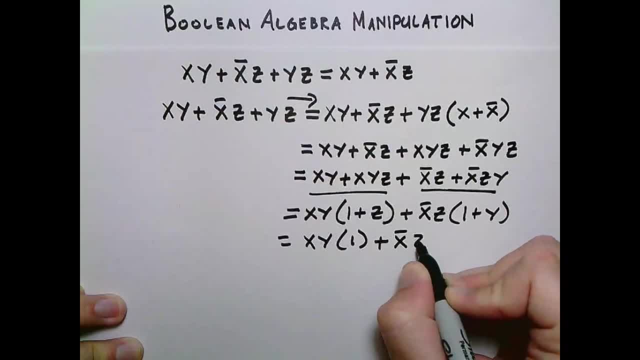 and 1, or not X and Z and 1, and anything and-ed with 1 is just itself. so the result is X, Y or not X, Z, which is what we were trying to get to. 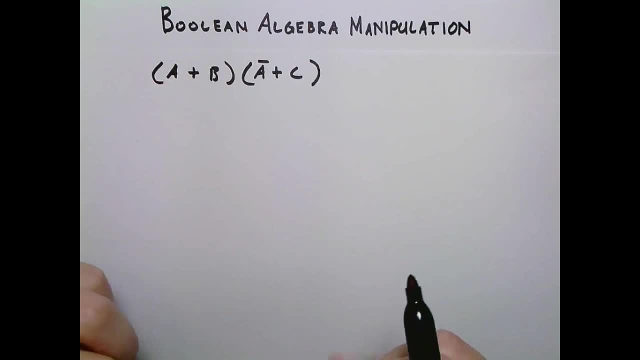 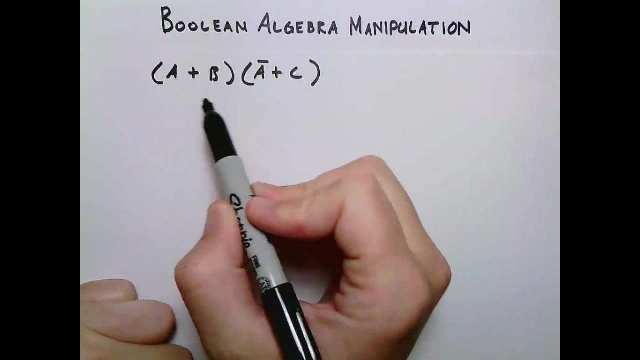 So worked out pretty cool, Alright. so let's do one last example, And this example is going to illustrate some- two things that are kind of interesting. The first: you'll notice that this Boolean expression, or Boolean equation, is in a different form than we're used to, right? 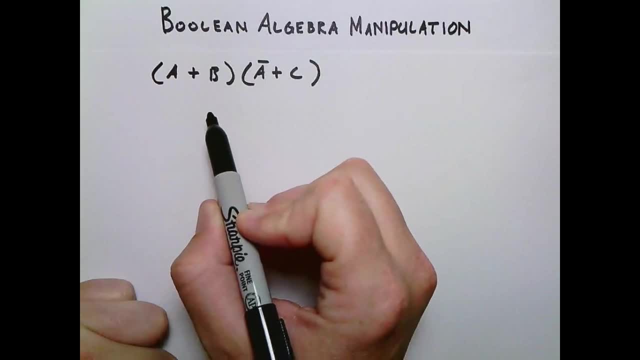 We're used to seeing things in what's called um sum of products form, where we have something in something or something in something or something or something. This is in what's called product of sums form, and we typically don't like it. 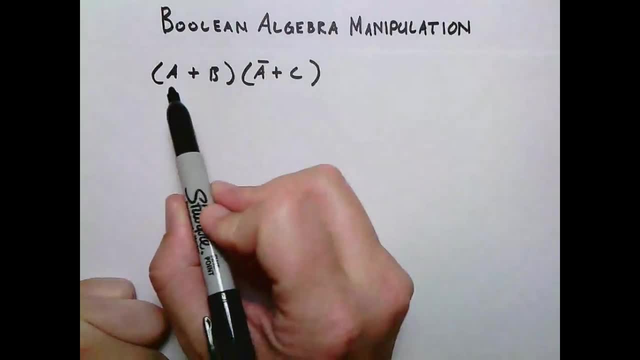 And we'll talk about why We don't like it in a later lesson. But let's see if we can sort of get it out of this form and then simplify it just a little bit. So the first thing that's kind of cool is in Boolean algebra. 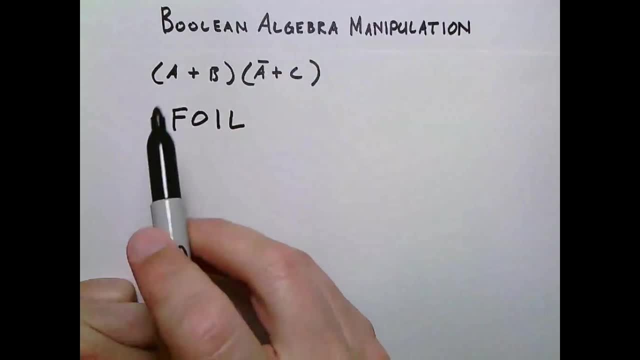 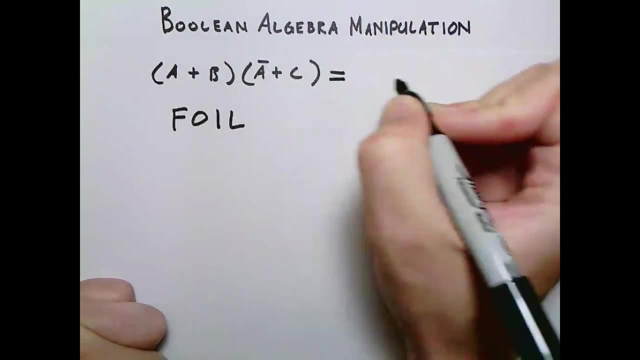 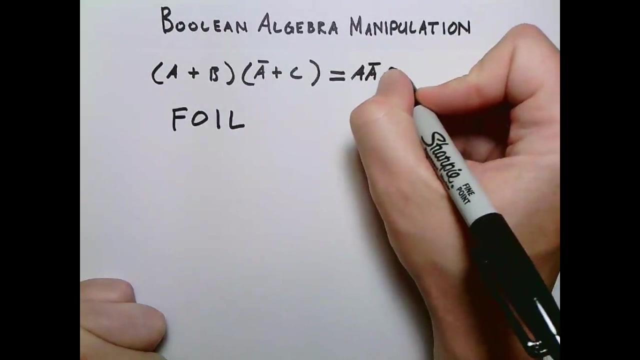 the concept of FOIL, which you should remember from high school algebra class, still applies right First, outside, inside last to get it from this form back into sum of products form. So let's do that. We're going to have A or not A. excuse me, A and not A. 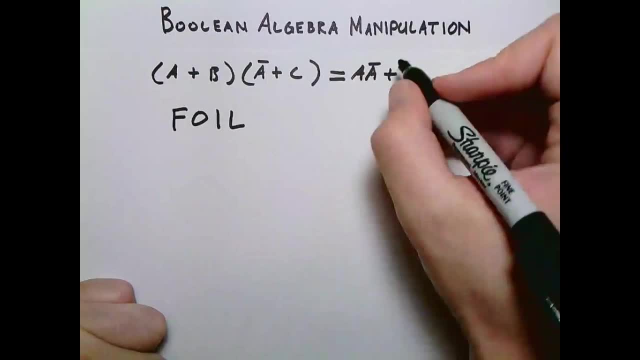 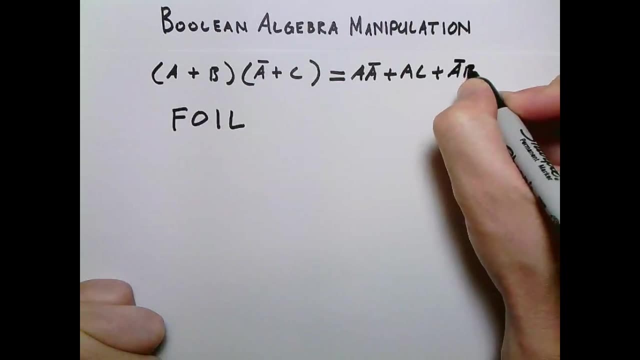 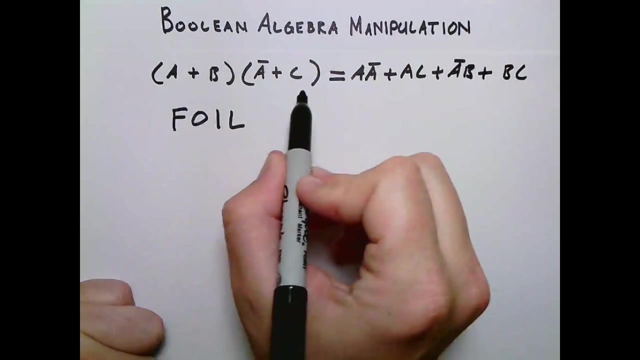 or um outside A and not A and C, or inside not A and B or B and C. So there we go. We've gone from product of sums form into sum of products form. Now let's do a little bit of simplification. 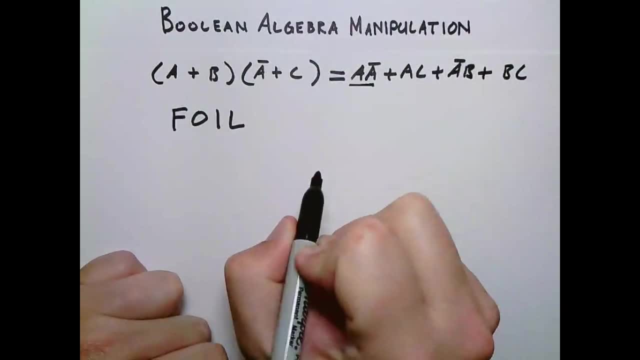 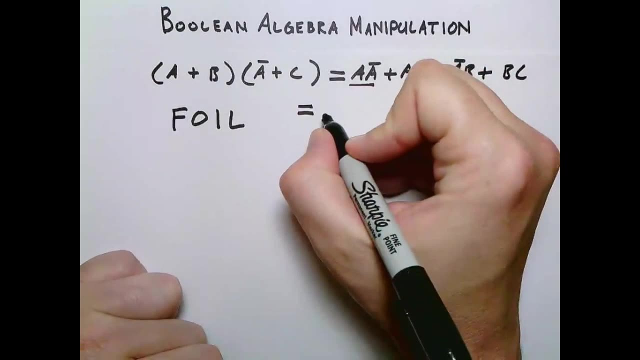 And the first thing that should jump out is this guy right here. We've got A and not A, And we know from our identities lesson that anything anded with its complement is going to be zero, So those guys are going to cancel out.